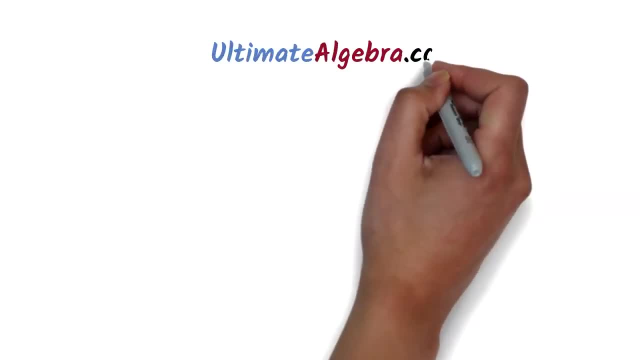 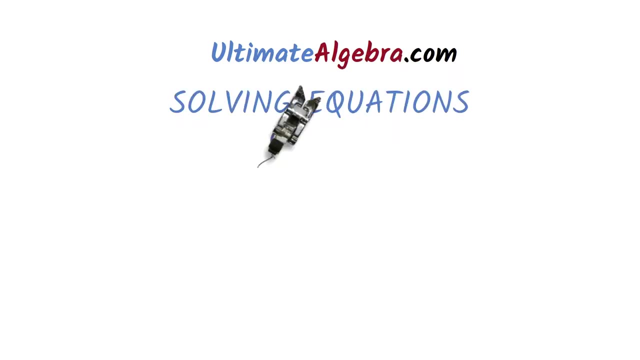 Welcome to another video from ultimatealgebracom. In this video, we will be looking at solving equations. This is by far the most important topic in math. Everything you'll do in math- whether it's division or graphs or whatever- is to aid you to solve equations. It's important. 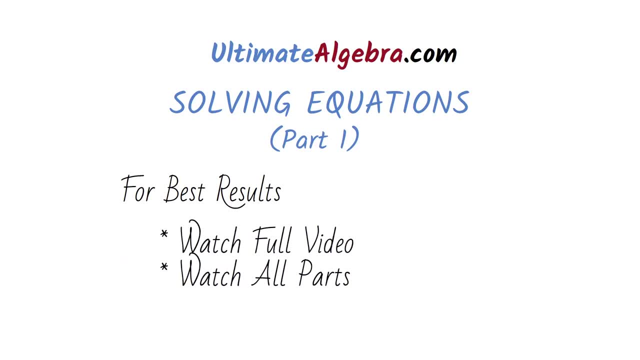 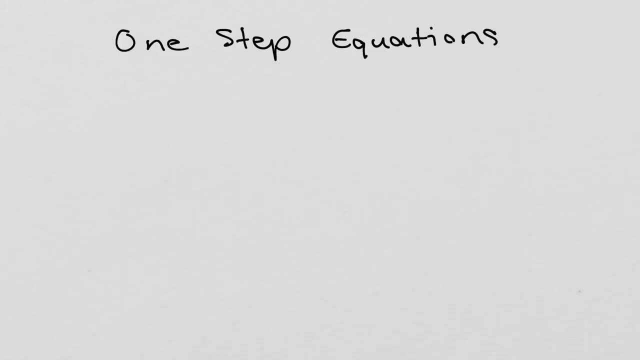 you watch the full video, because it's step-by-step, and also watch all subsequent videos, One-step equations. Let's look at an example: x plus 2 equals 5.. Solve for x. The idea of solving equations is to move everything with the x to the other side of the equation by performing the opposite. 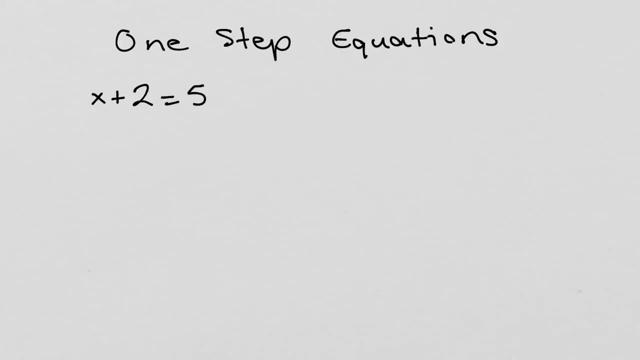 operation on it. We want only the x to be on one side of the equation. So here we want to move the plus 2 to the other side of the equation. We do that by performing the opposite operation on both sides of the equation. The opposite operation of addition is subtraction. 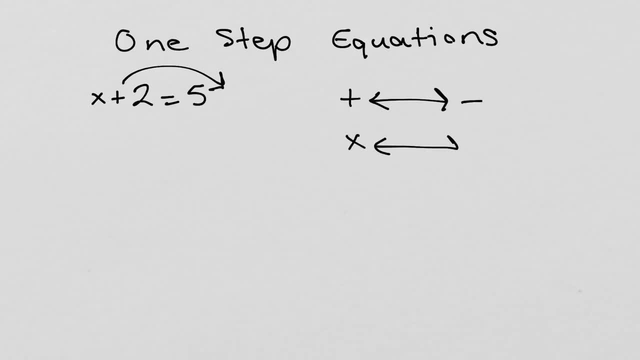 The opposite operation of multiplication is division. The opposite operation of exponent is root or radical. The opposite operation of addition is subtraction. So we will subtract 2 from both sides. Once the opposite operation is done, those two numbers simply cancel out. So here: 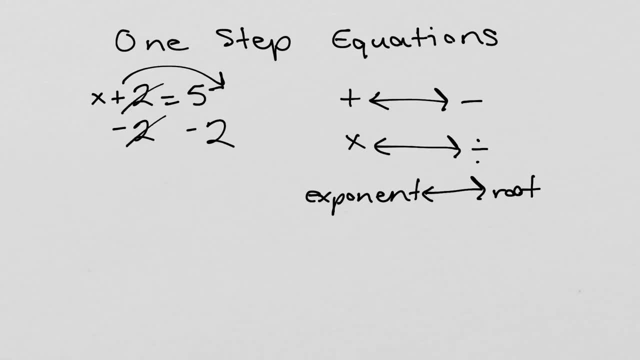 the two cancels out, 5 minus 2 is 3.. So x will be equal to 3.. Let's look at another example. So here the two cancels out equals 35. Solve for a Here again. we want to get rid of anything that is with the a. 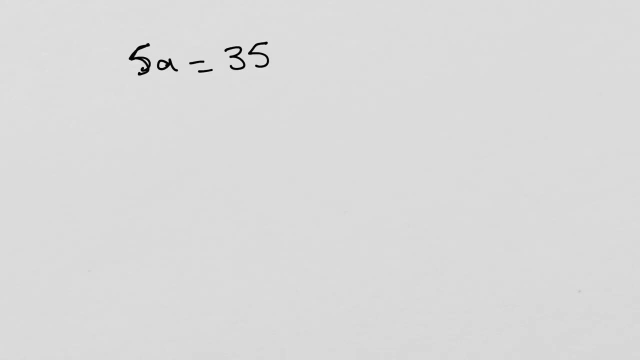 This means we have to get rid of the 5.. So 5a is the same as 5 times a. Since the 5 is multiplying, we will perform the opposite operation on it. We know that the opposite operation of multiplication is division. 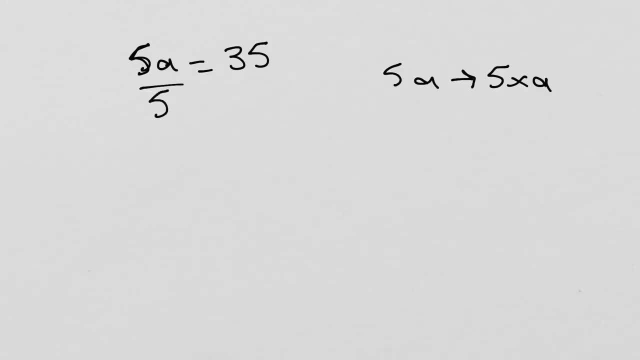 so we will divide both sides by 5.. Since we performed the opposite operation, we can say that the 5 will cancel out. Now, 35 divided by 5 is 7.. So a equals 7.. Now try these questions and leave your answers in the comments section. 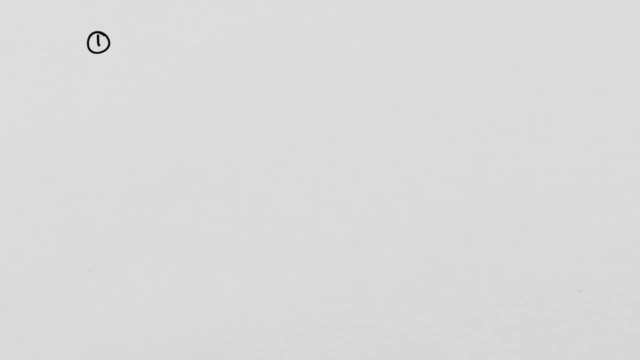 Number 1. Solve for x and x. x over 9 equals 3.. Number 2. Solve for x and x minus 6 equals 12.. Number 3. Solve for b and 3b equals 18.. Remember, you are just performing the opposite operation on both sides. 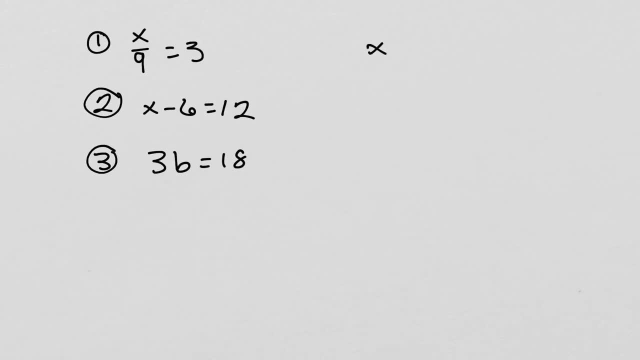 So in the first question, for example, you will have to multiply both sides by 9.. The 9 is dividing. We will perform the opposite operation on both sides of the equation, So you will have to multiply both sides by 9.. The 9 will cancel out, since we performed the opposite operation on it. 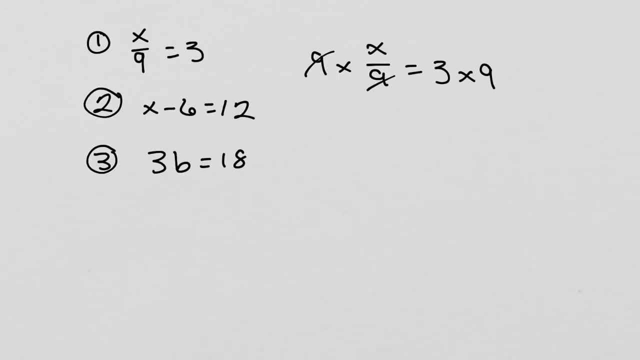 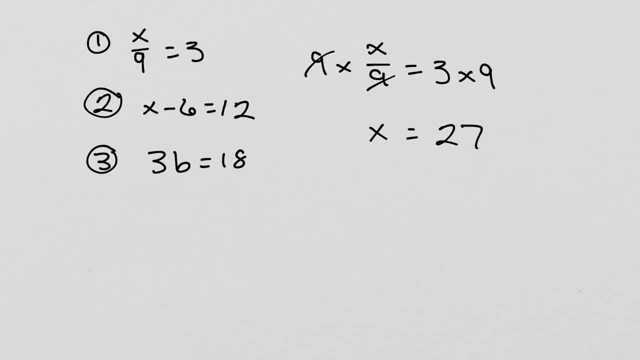 I will leave the next two questions to you. In the examples we've done so far, we needed to perform only one operation to solve the questions. So for our first example, we just did subtraction. For our second example, we just did division. 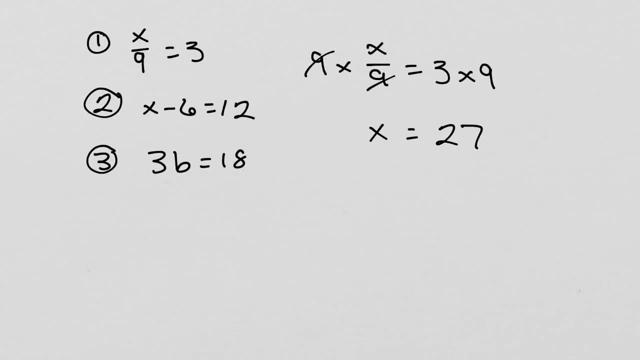 And for this one, we just did multiplication. That is why they are called one-step equations, Two-step equations. However, you can move these equations forward and backwards. Some of you also may need to do multiplication. This kind of thing is problem solving. 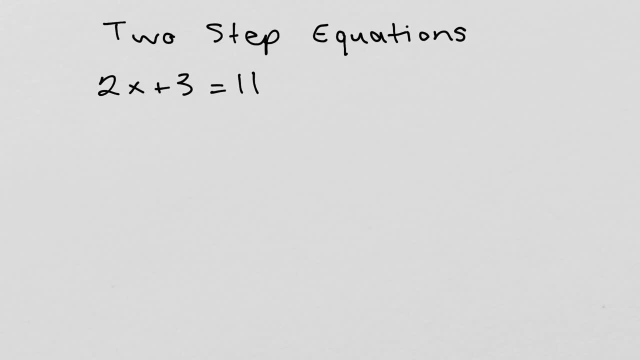 So those are Two-step and Multiplication equations. Then we have multiplication, We have two-step equations or multiplication, And then again we have multiplication. so we have one-step and multiplication. in this case The multiplication can be done randomly by increasing the number of boxes. 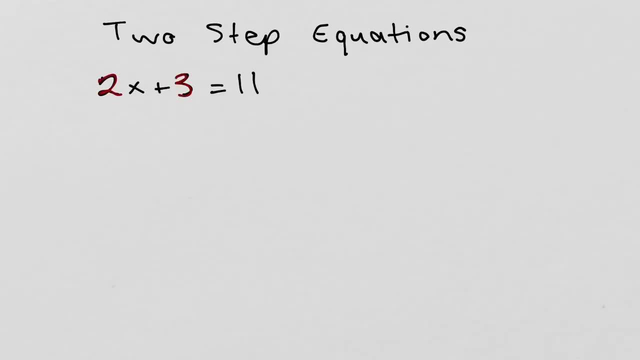 But it can also be efficiently plusieurs way. so you can either do multiplication creatively or do multiplication randomly. Remember we said 2x is the same as 2 times x. When there are more than one operation, we use the idea of the reversal of the order of operations to know which one to get rid of first. 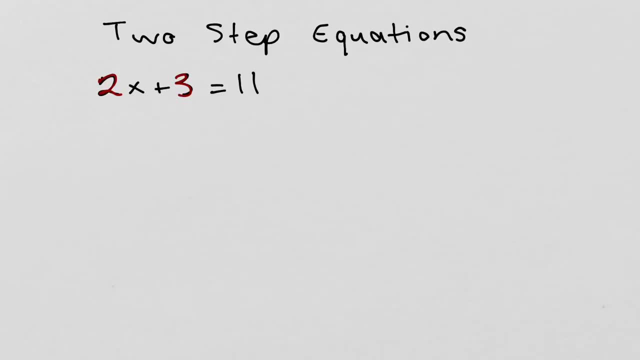 So here is the order of operation. If you are not familiar with the order of operation, we've put a link in the description for you to master it. It's important that you watch it. Knowing the order of operation will make solving of equations super easy. 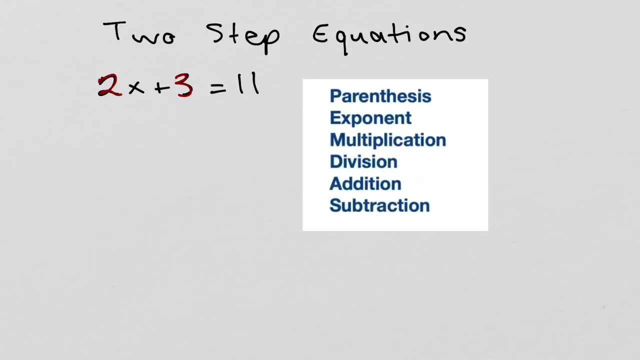 We can see that in the reversal of the order of operation we have addition first and multiplication second, So we will get rid of the plus 3.. We get rid of the plus 3 by performing the opposite operation on it, So we will subtract 3 from both sides. 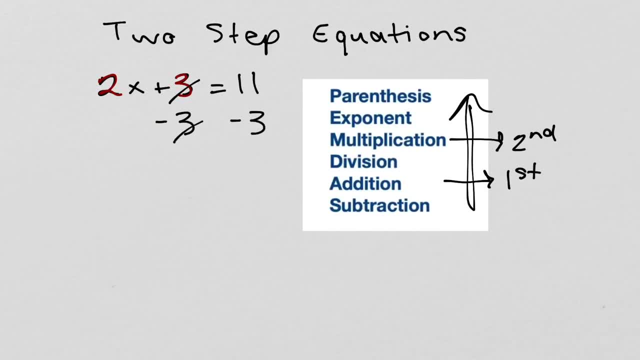 The 3 will cancel out. 11 minus 3 is 8, so we have 2x equals 8.. Next, we will get rid of the multiplication by dividing both sides by 2.. Since we have 2x, we will get rid of the multiplication by dividing both sides by 2.. 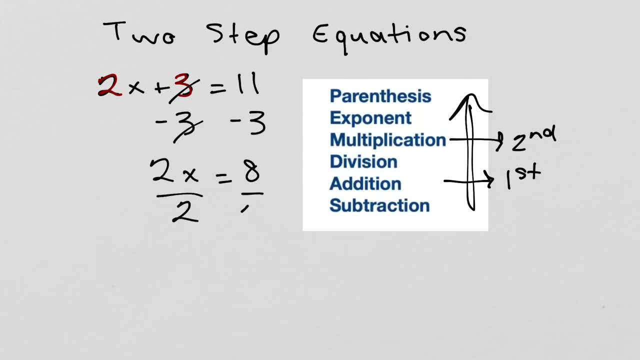 So we have 2x equals 8.. Since we have 2x, we will get rid of the multiplication by dividing both sides by 3.. This division is the opposite of multiplication. The 2 will cancel out. 8 divided by 2 is 4, therefore x equals 4.. 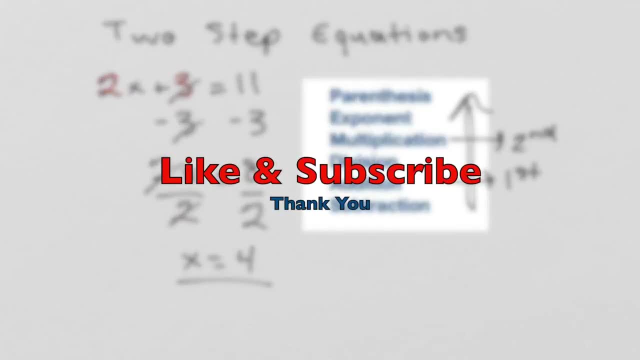 Before we take more examples, we want you to do us a huge favor by liking this video. This is really the best thing you can do to encourage us to make more videos. If we don't know you like the videos, we won't have any reason to be satisfied. 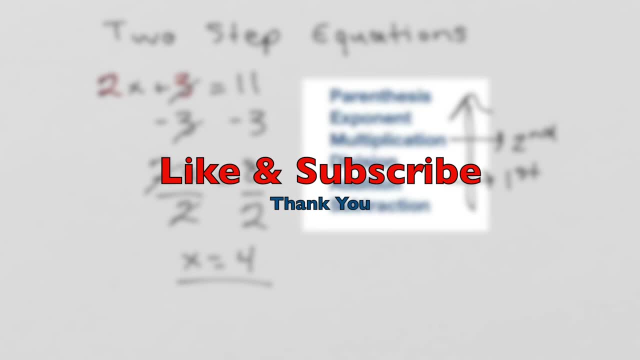 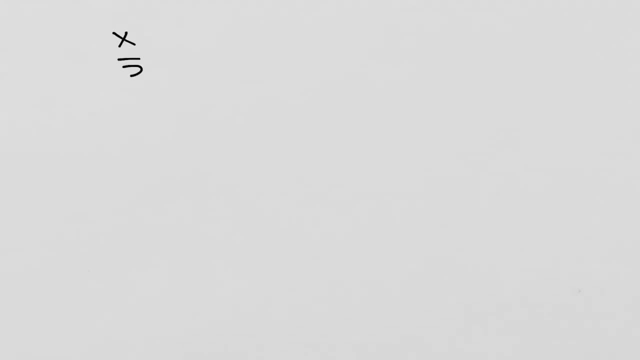 suppose more. Okay, let's take our next example. Solve for x and x over 3 minus 4 equals 6.. We want to get rid of all the numbers attached to the x so we can have the x alone on one side of the equation. To achieve this, we know that we must get rid of the divided by 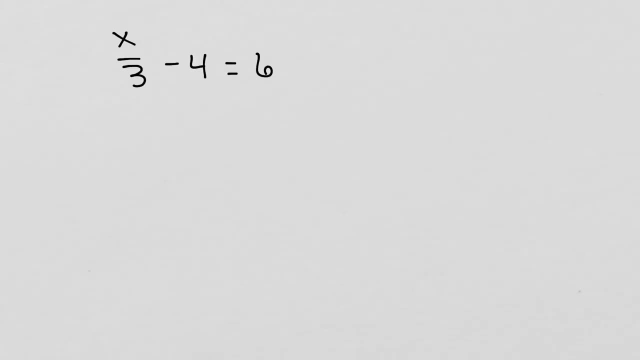 3 and the minus 4.. Let's write our order of operations, Please. you don't need to be writing the order of operations in your solutions. at school, We are using it for teaching purposes. We are using a reversal of the order of operations. 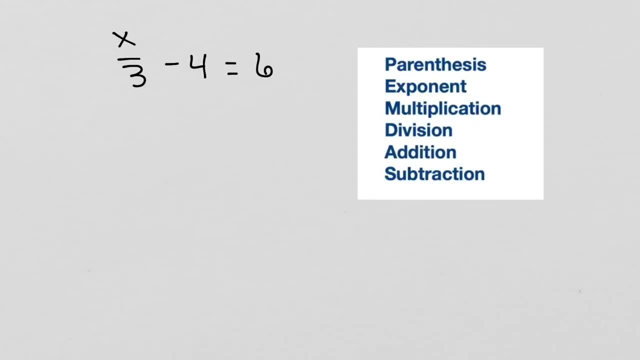 so we are working from the bottom up. We will see that the order of operations, for the first time that we get rid of all the that in this form, we must do subtraction first and division second. To get rid of the minus 4, we must perform the opposite operation on both sides of the equation. 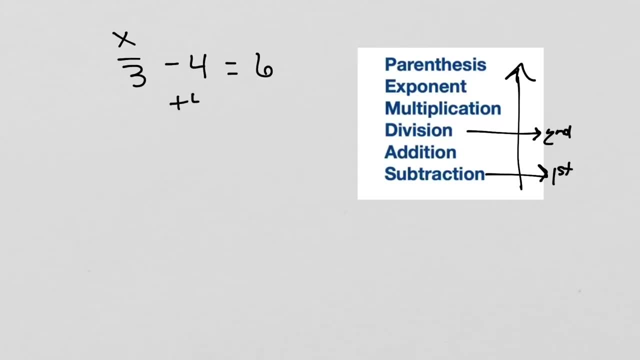 so we will add 4 to both sides. The 4 will cancel out. 6 plus 4 is 10.. We now have x divided by 3 equals 10.. Next we will get rid of the divided by 3.. We do. 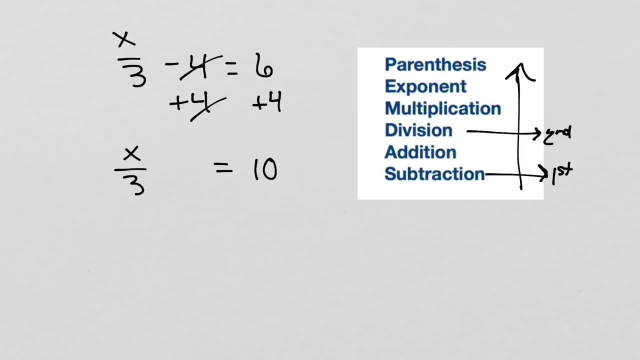 this by performing the opposite operation on both sides of the equation. So we will multiply both sides by 3.. The 3 will cancel out 10 times. 3 is 30. therefore x equals 30.. In most instances for two-step equations you will work out your addition or. 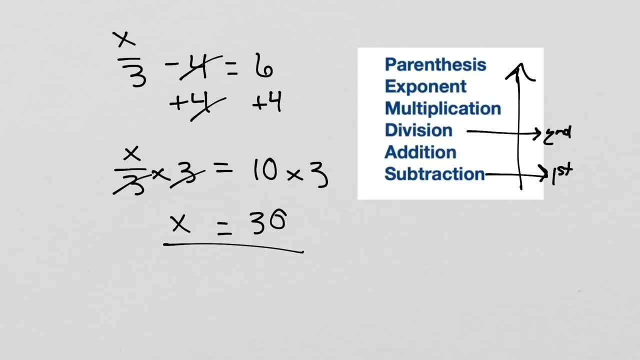 subtraction part first, then you will work out your multiplication or division part next. Please, this is not always the case. topics like this requires practice, practice, practice. You want to be so good at it that you don't need to use the reversal of the order of. 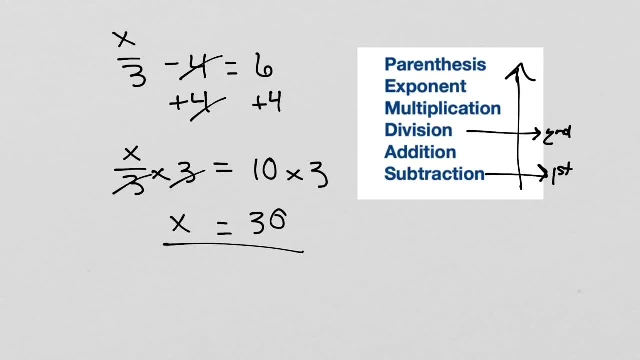 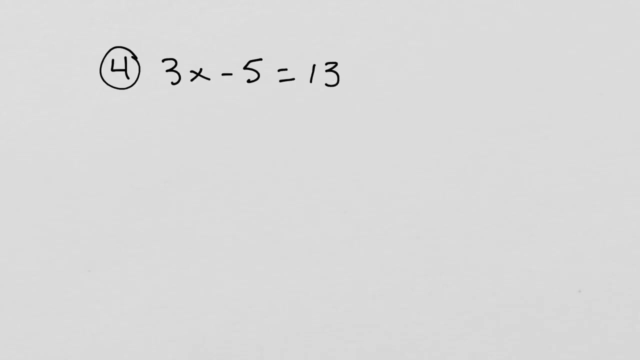 I operations anymore. You see a question and you just know which one to do, first and second. You can get more practice with the link in the description. Try the following and leave your answers in the comment section. Number four: 3x minus 5 equals 13.. Solve for x Number five. 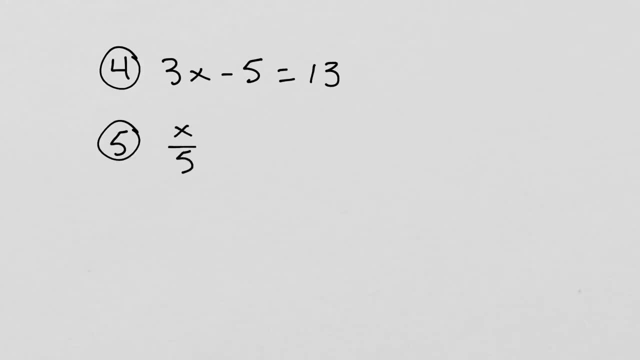 x over 5 plus 3 equals 8.. Solve for x. Most confusing two-step equations. Two-step equations that require distribution or has an operation in parentheses is the one most students get confused with. In fact, not all math teachers agree that this is a proper two-step equation, but it is. Let's look at. 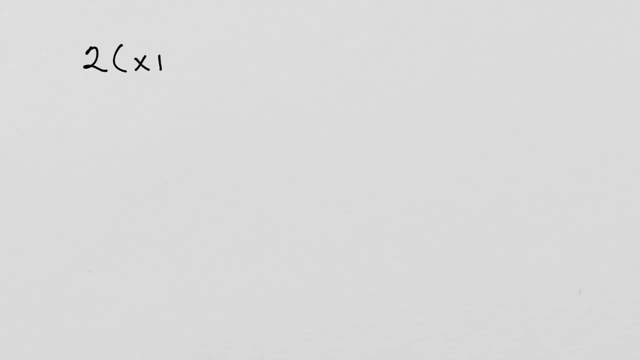 a two-step equation that requires distribution or has an operation in parentheses. Two parentheses: x plus 5 equals 16.. We will solve it two ways. Method one: we will first distribute the two. The two will multiply everything in the parentheses, So the two. 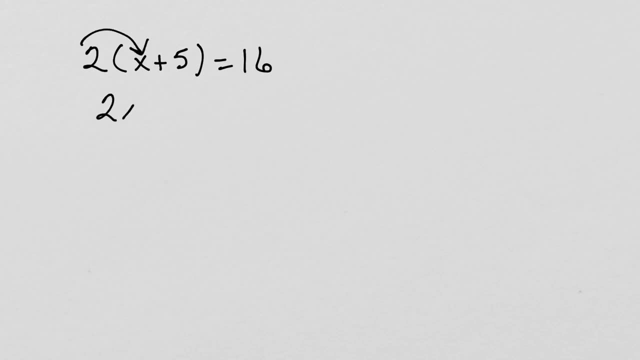 will multiply the x to get 2x, plus the two will multiply the 5 to get 10.. We have: 2x plus 10 equals 16.. We can see that we have a familiar two-step equation. Let's write our order of operation. 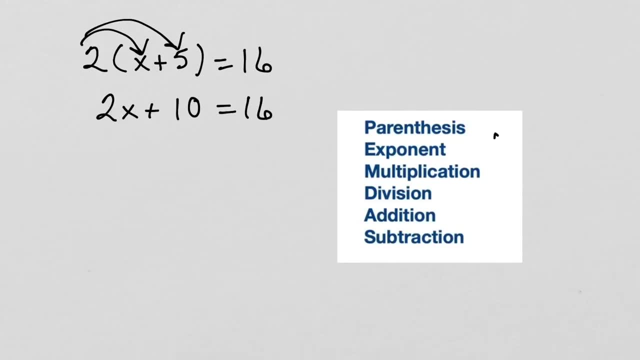 Using the reversal of the order of operation. we will do the plus 10 first and then the times 2. We get rid of the plus 10 by subtracting 10 from both sides. The 10 will cancel out. 16 minus 10 is 6, so we have 2x equals 6.. 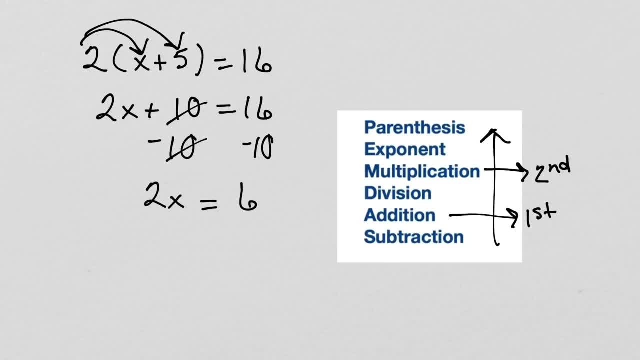 Next, we will get rid of the times 2 by dividing both sides by 2.. The 2 will cancel out 6 divided by 2 is 3, so x equals 3.. Here you realize that we did an extra step of distribution. 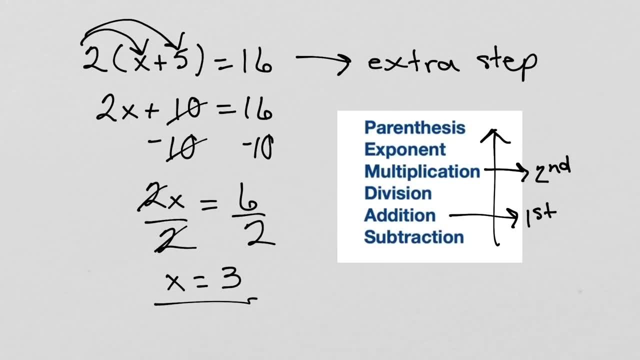 before we could apply the two-step equation. You can solve it this way if it's easy for you, but that's not the best way to solve it. Let's look at method 2.. For the purpose of teaching, we're going to break this down. 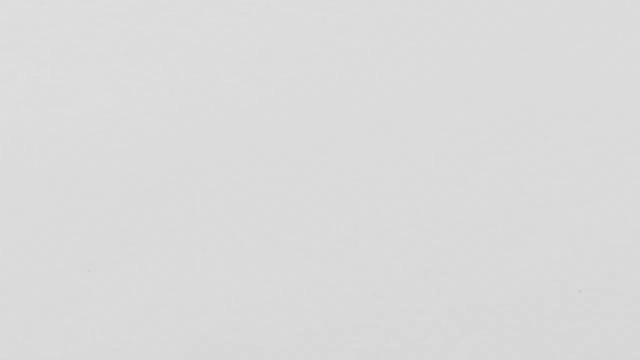 But your goal is to be familiar with questions like this so that you don't need all this breaking down and thinking to solve it. Let's write the order of operation again. In the order of operation, parentheses are performed first. When we say parentheses are performed first, we're saying that parentheses are performed. 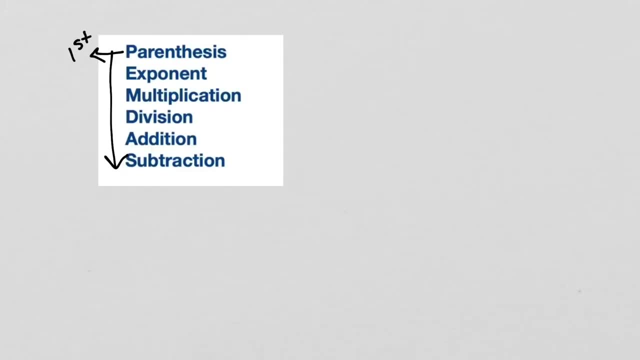 first. What we actually mean is that the operation in parentheses is performed first. So if we have 3 times parentheses- 2 plus 4, then we will perform the 2 plus 4 first because it's in parentheses. So basically, we perform the addition operation first because it's in parentheses. 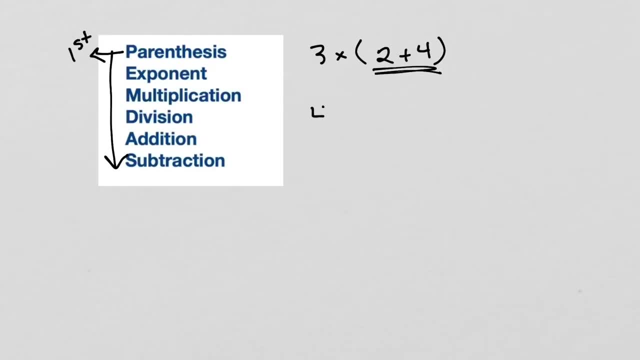 Similarly, if we have 4 plus 6 parentheses, 2 plus 4, we perform the addition operation first because it's in parentheses: times 7, exponent 3.. We will perform the 2 times 7 first because it's in parentheses. So we perform the multiplication operation. 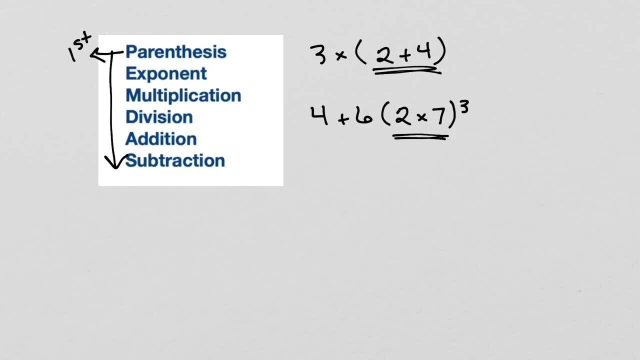 first because it is in parentheses. Now, since we know that equations are solved with the reversal of the order of operation, it means that we will solve the operation in the parentheses last. With that in mind, let's look at our question 2, parentheses x plus 5. 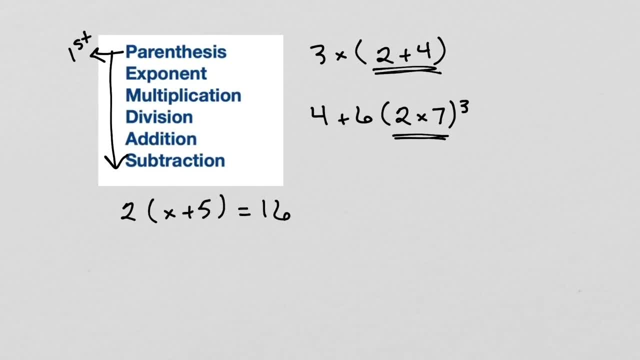 equals 16.. Remember, 2 parentheses x plus 5 is the same as 2 times parentheses x plus 5.. Here, since the x plus 5 is in parentheses, we will call it a parentheses operation. So we have multiplication operation and a parentheses operation. 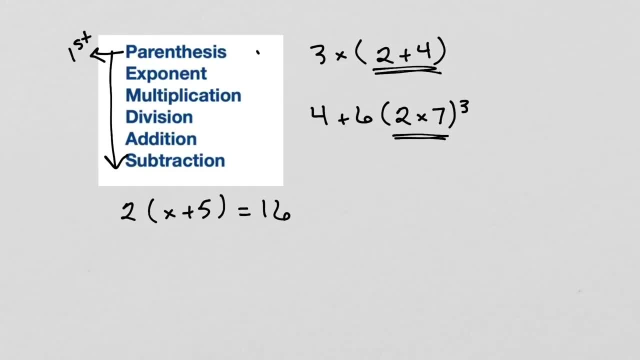 Using the reversal of the order of operation, we will solve the multiplication operation. We will do the multiplication first and parentheses last. We get rid of the times 2 by dividing both sides by 2.. The 2 will cancel out. 16 divided by 2 is 8.. 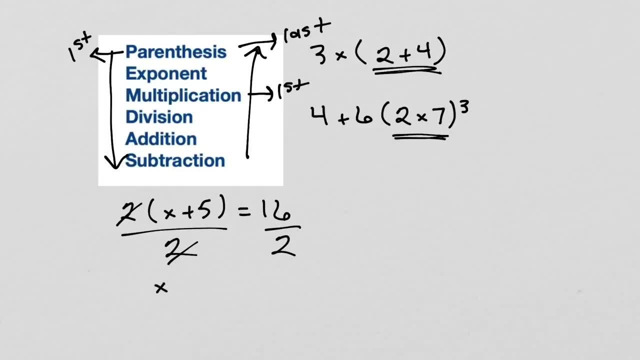 Now we can remove the parentheses to get x plus 5 equals 8.. Once you're about to perform the operation in parentheses, you can remove the parentheses. We will get rid of the plus 5 by subtracting 5 from both sides. 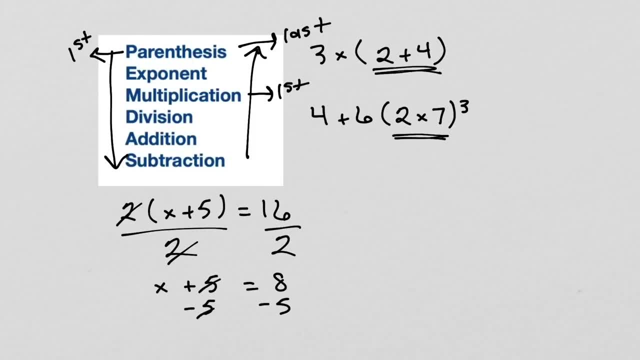 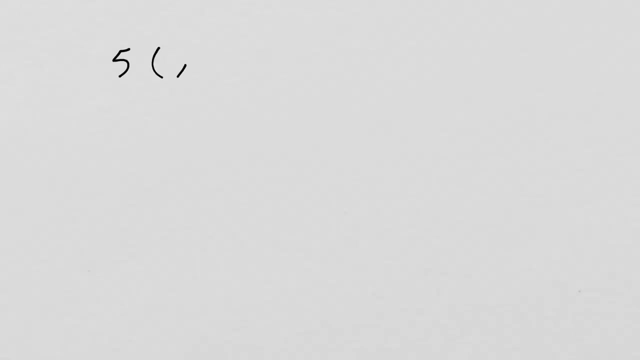 The 5 will cancel out. 8 minus 5 is 3.. Therefore, x equals 3.. You will realize that here we did only two steps. Therefore, this is a true two-step equation. Try this question: 5 parentheses. x minus 7 equals 55.. 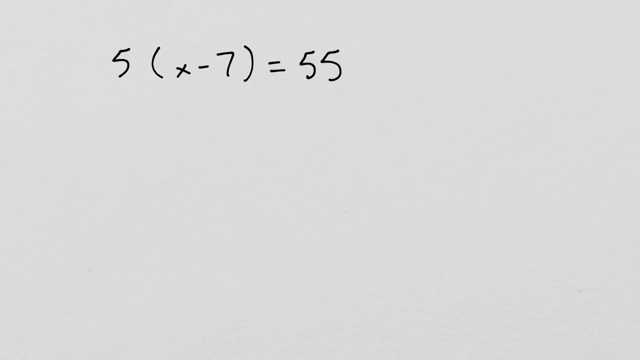 Solve for x. Pause the video and try it first. We can see that we have a multiplication operation and an operation in parentheses. Using the reversal of the order of operation, we will do the multiplication operation first and then the operation in parentheses. We remove the times 5 by dividing both sides by 5.. 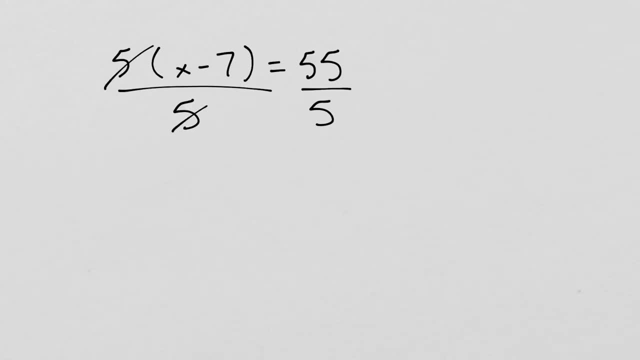 The 5 will cancel out. 55 divided by 5 is 11.. So now we have: x minus 7 equals 11.. Again, once you are about to perform the operation in parentheses, you can remove the parentheses To remove the negative 7, we will add 7 to both sides of the equation. 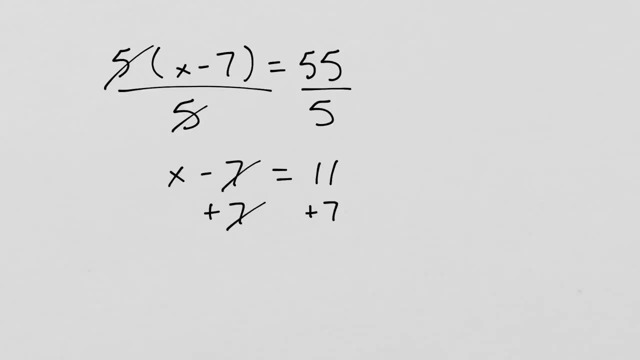 The 7 will cancel out. 11 plus 7 is 18.. So x equals 18.. Let's look at parentheses: x minus 6 over 4 equals 6.. Please pause this video and try it before you watch our solution. 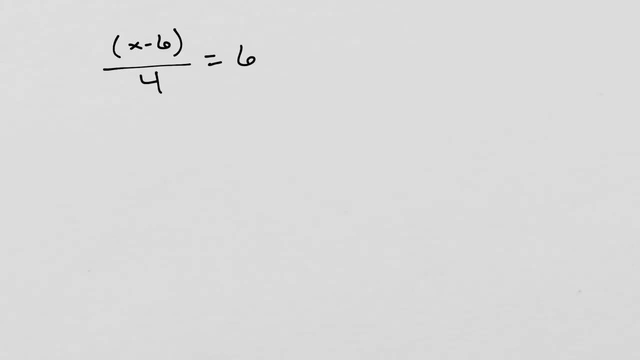 Here we have a division operation and an operation in parentheses. Let's write our order of operation From the reversal of the order of operation. we have to do division first and parentheses less. We get rid of the divided by 4 by multiplying both sides by 4.. 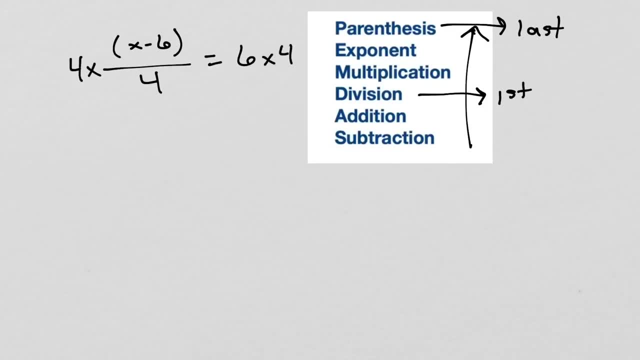 Okay, The 4 will cancel out. The 4 will cancel out. 6 times 4 is 24.. Now we can remove the parentheses to half. x minus 6 equals 24.. We get rid of the minus 6 by adding 6 to both sides. 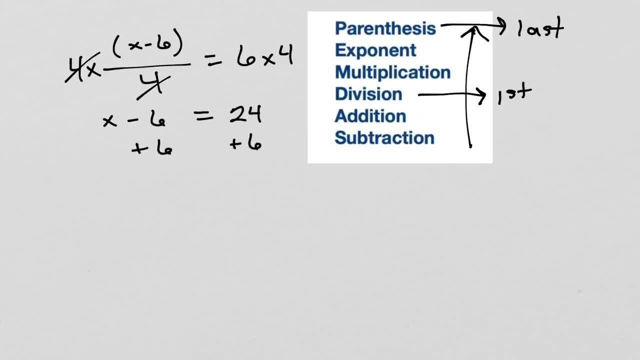 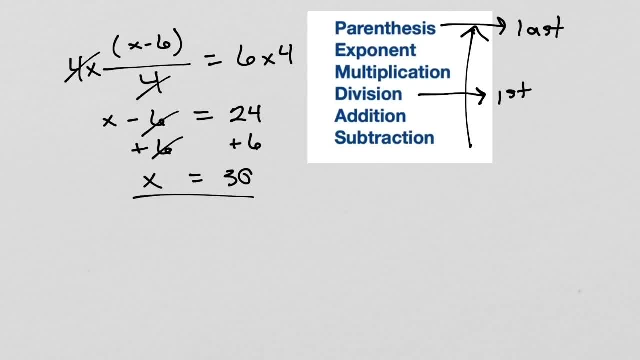 When it comes to division, the parentheses is usually not written, So parentheses x minus 6 over 4 will be simply written as x minus 6 all over 4.. When you say number dividing two or more numbers, this way parentheses is implied. So 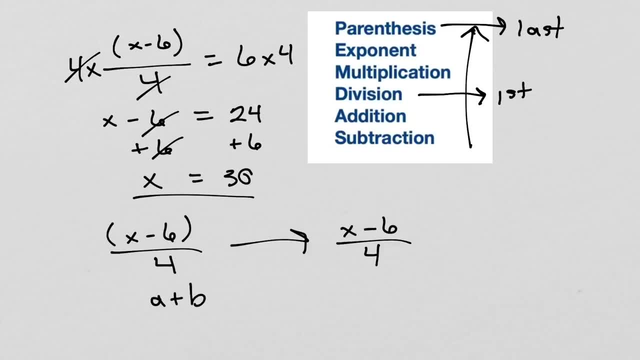 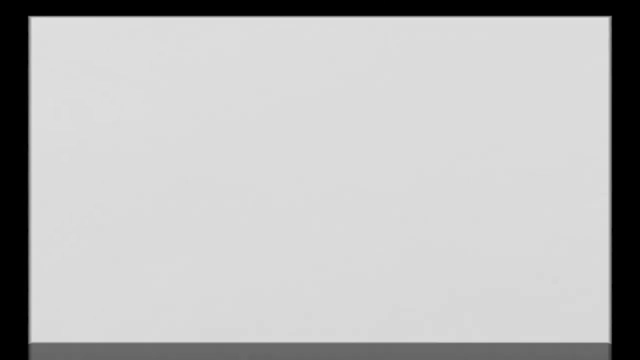 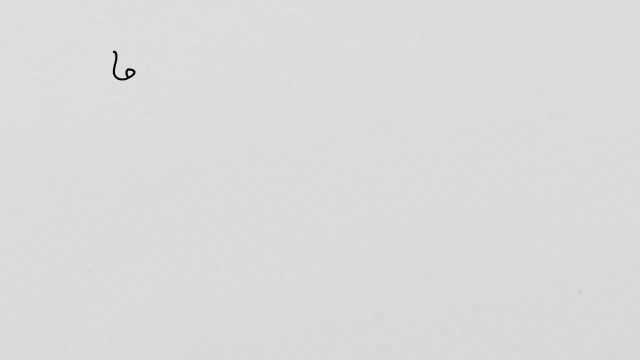 a plus b plus c equals 30.. All over 5 is the same as parentheses a plus b plus c, all over 5.. Please try these and leave your answers in the comment section, Number 6.. 3 parentheses x minus 5 equals 21.. 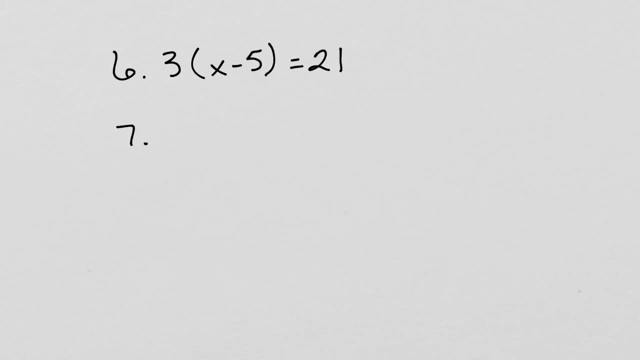 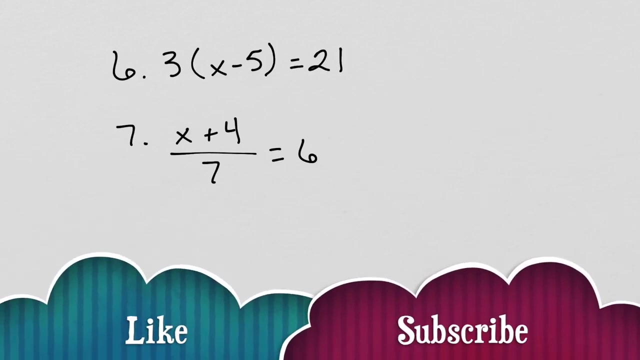 Number 7.. x plus 4, all over 7 equals 6.. We will end this video here. Please go over it as many times as needed. This topic is just too important. Master the use of the reversal of the order of operation, because we will be using it in the next video.